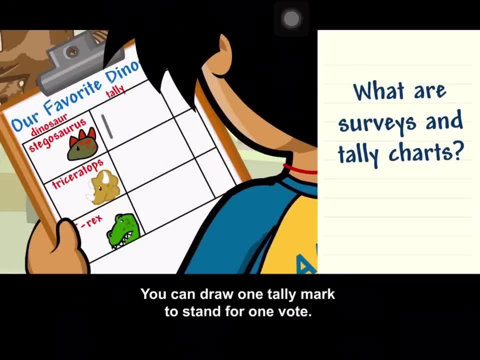 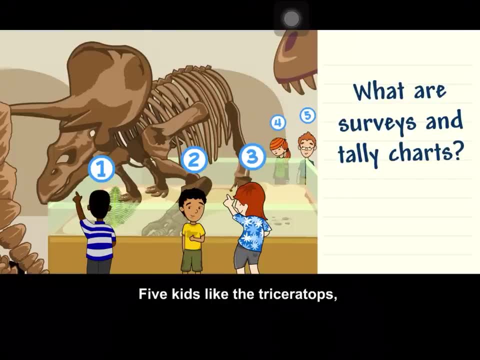 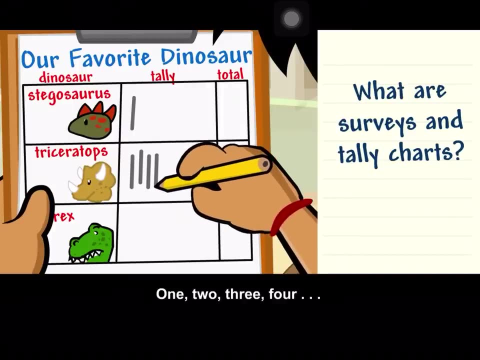 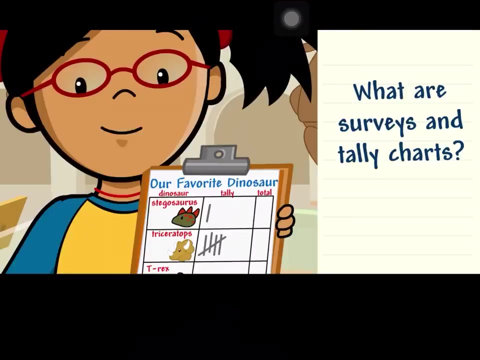 You can draw one tally mark to stand for one vote. Five kids, like the triceratops. So I'll draw five tally marks in that row: One, two, three, four. The fifth mark is drawn across the other four. Well, when you group the tally marks by fives, you can count by fives. 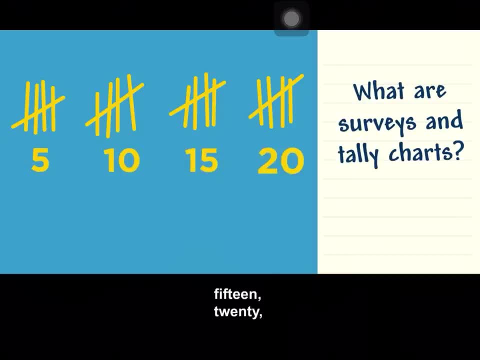 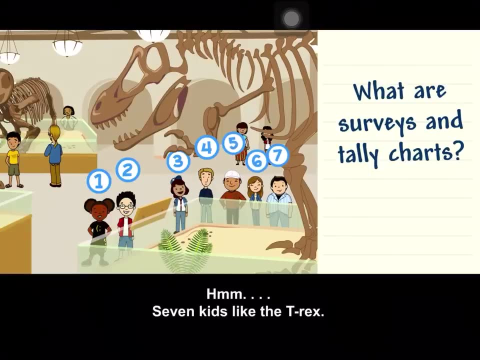 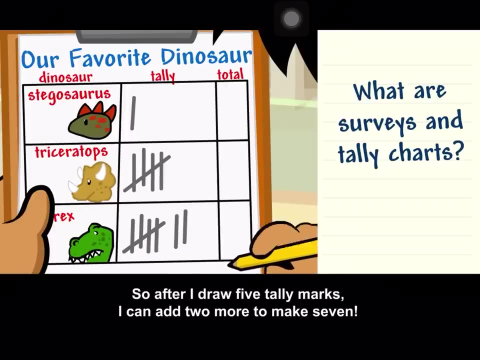 Five, ten, fifteen, twenty Sets of fives are easier to count. Hmm, Seven kids like the t-rex. So after I draw five tally marks, I can add two more to make seven. Oh right, I forgot to vote. my favorite dinosaur is the triceratops. 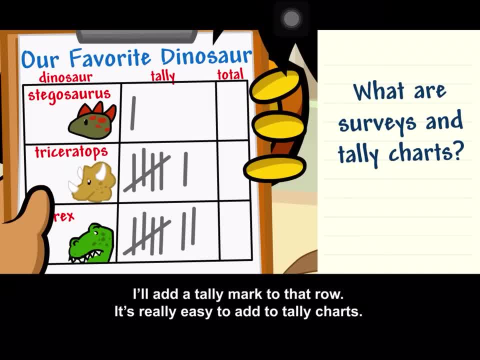 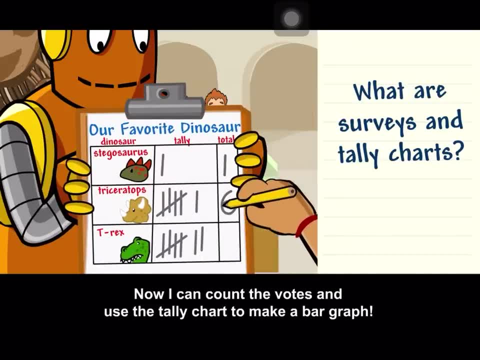 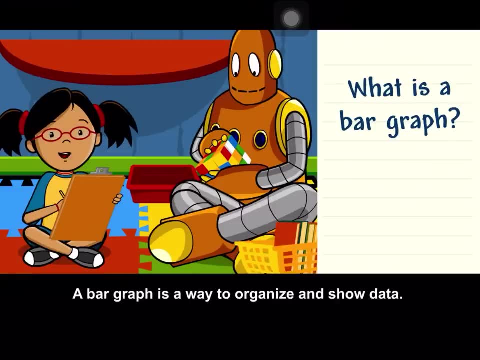 I'll add a tally mark to that row. It's really easy to add to tally charts. Now I can count the votes and use the tally chart to make a bar graph. What is a bar graph? A bar graph is a way to organize and show data. You can write the categories on the bottom, The. 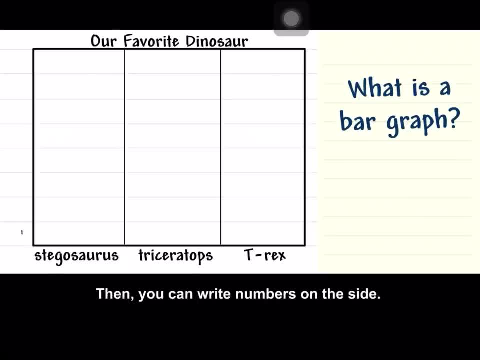 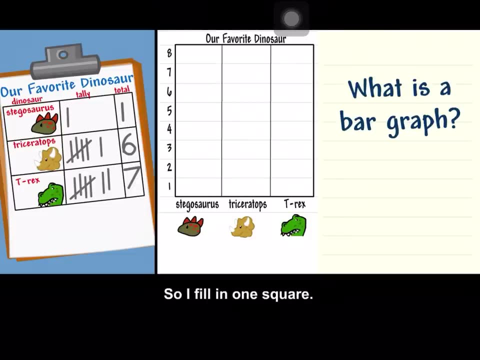 three dinosaurs are the categories. Then you can write the numbers on the side. The numbers in our bar graph show how many people voted for each dinosaur. Let's see: One student liked the Stegosaurus the best, so I fill in one square. Six people voted for the Triceratops, so I color in six squares. 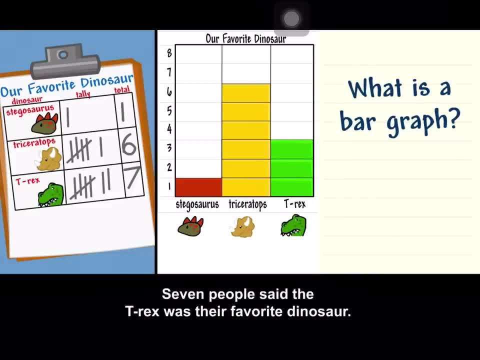 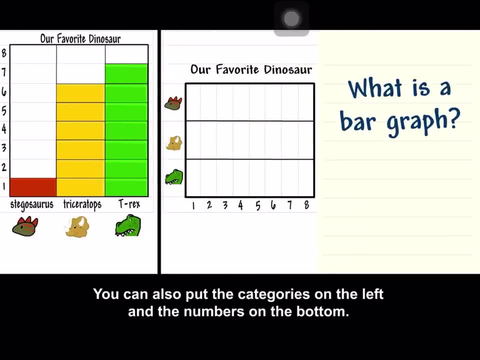 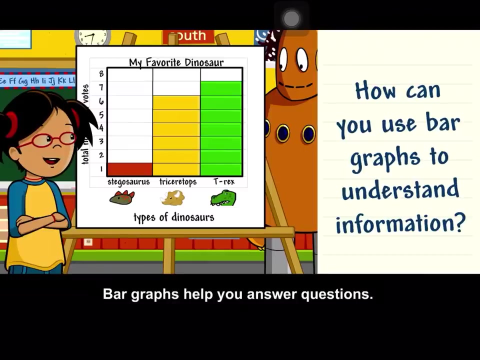 Seven people said the T-Rex was their favorite dinosaur. You can also put the categories on the left and the numbers on the left. You can display the same information in a different way so you can understand it better. How can you use bar graphs to understand information? Bar graphs help.